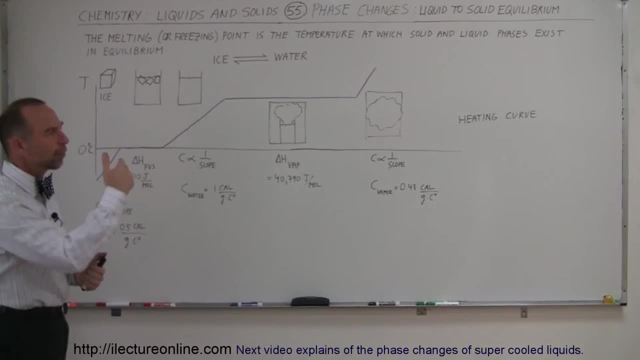 we have a flat line. So what does that really represent? Well, let's go over what the heating curve really is. A heating curve is kind of representation of if you were to add, for example, energy to whatever you start with. Let's say, we start with a block of ice at maybe. 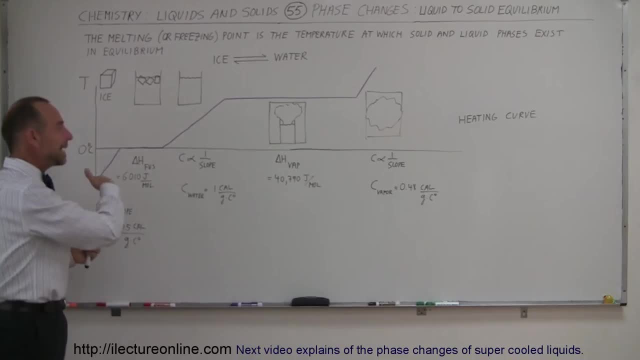 minus 50 or minus 100 degrees centigrade and you start adding heat to that block of ice at a, say, a constant pace, the same amount of energy per unit time. then what would happen? Well, initially the ice would gain temperature. It will increase in temperature until the ice reaches the 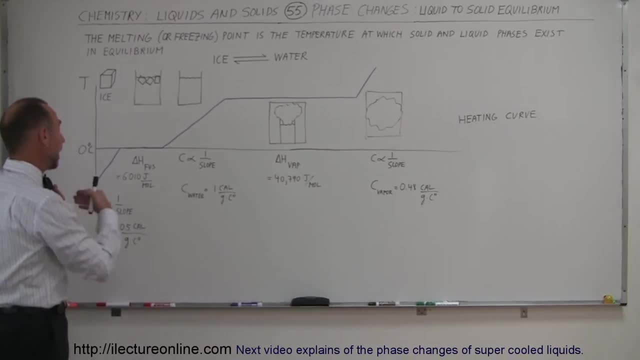 temperature of zero degrees centigrade. At that point, continuing to add the same amount of heat at a constant rate, the temperature would no longer go up. The temperature would stay the same at zero degrees centigrade, and the ice would then begin to melt, Slowly but surely. 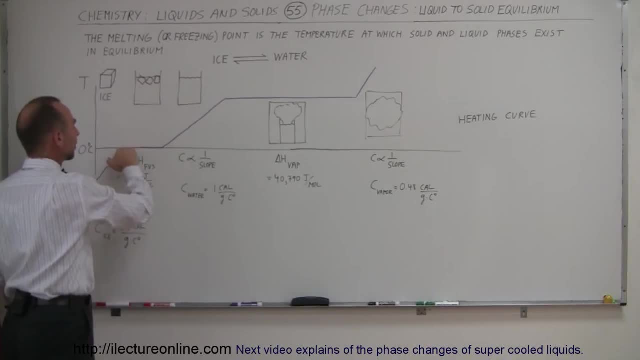 the ice melts. the ice melts, the water would not gain any temperature. the ice would stay at zero degrees centigrade until. If you then continue to add heat at a constant pace, then the water begins to heat up. Notice that the rate at which ice heat up is greater than the rate at which water heats up with the same. 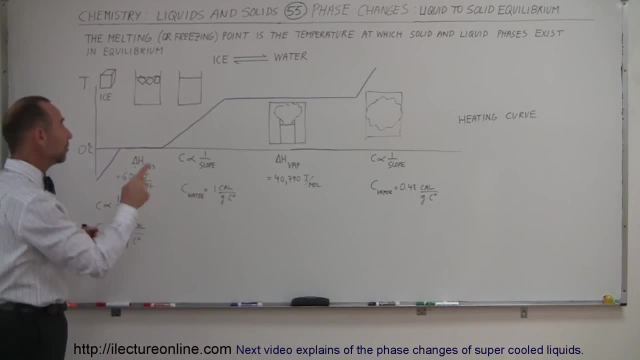 amount of heat added per unit time. The reason for that is that the specific heat of ice is smaller and the specific heat of water is greater. So if the specific heat is greater, that means you need more energy to make the temperature go up. So you can see C, the specific heat of water is. 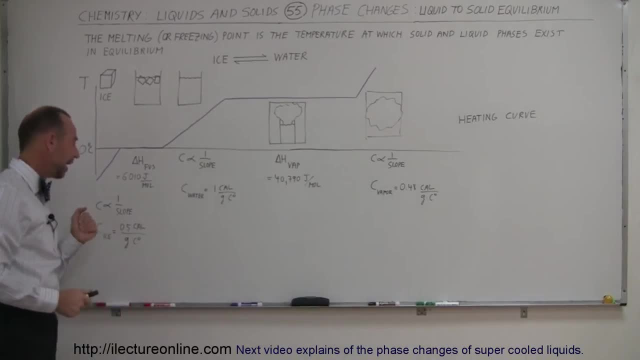 one calorie per gram per centigrade degree. For ice, it's only only about half that much. So you see, then, that means that the slope here is twice as steep as the slope over there. In other words, the specific heat is inversely proportional to the slope. 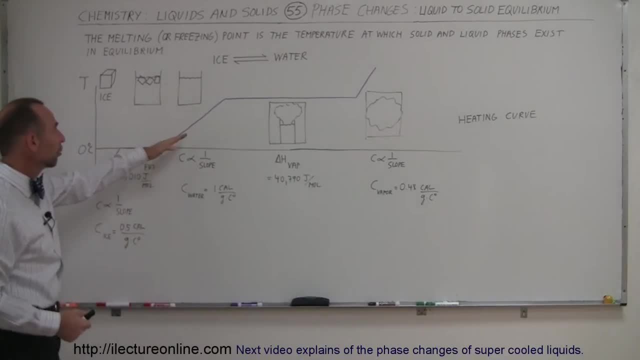 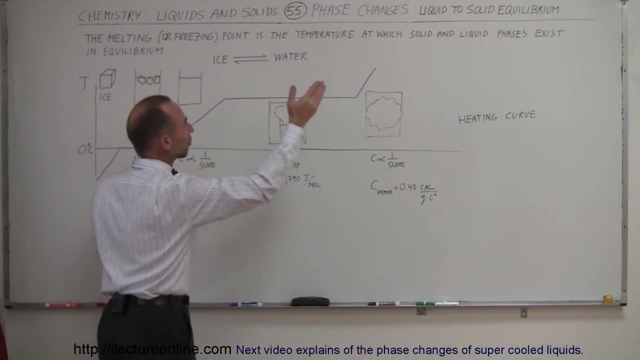 Make the slope bigger, smaller C. Make the slope smaller, bigger C. So they're inversely proportional. So that will then continue. Now, even though we're here talking about the liquid, that's all equilibrium. there's another point at which there's an equilibrium phase, that is between: 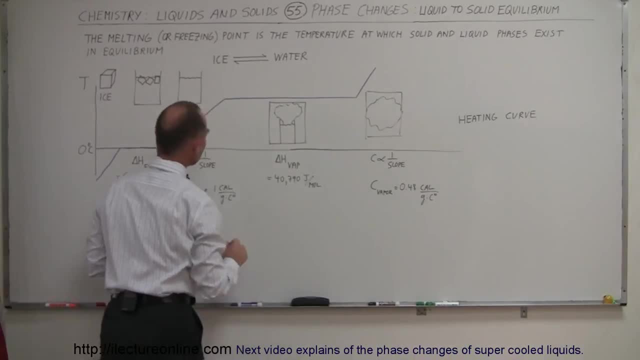 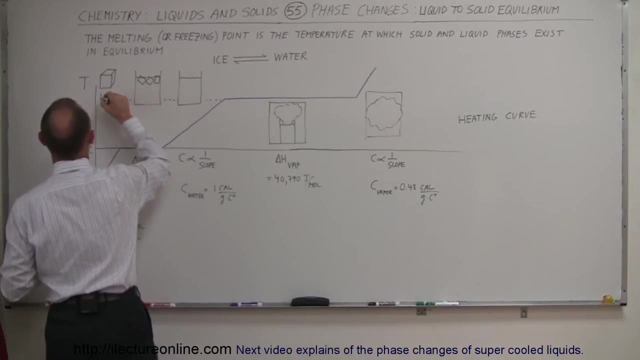 vapor and liquid. That would happen right here, Notice. the water would eventually reach a temperature of 100 degrees centigrade. So let me draw a line straight across here. There we go. So this would be 100 degrees centigrade at one. 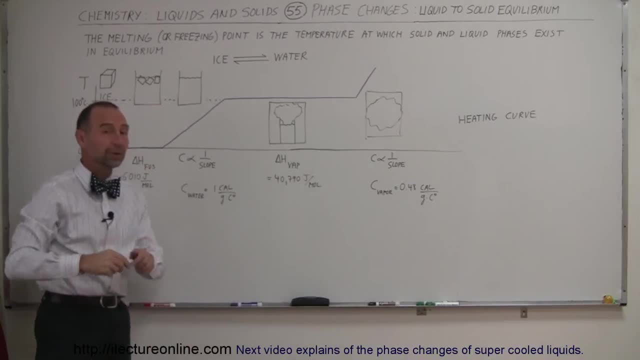 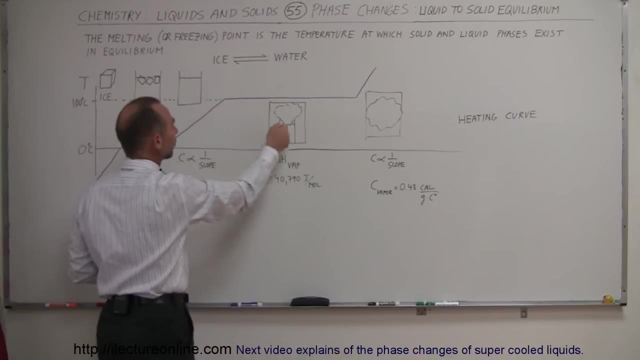 atmosphere, and that's when water begins to boil. Water will not heat up any more beyond 100 degrees centigrade. Any additional heat added to the water will then convert the water into steam, So I'll try to depict that here. Here's a little beaker of water. You add more heat. 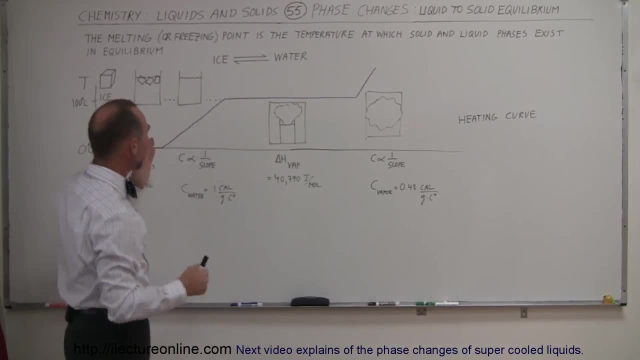 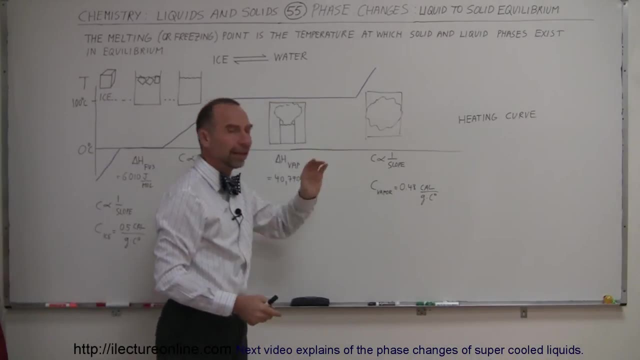 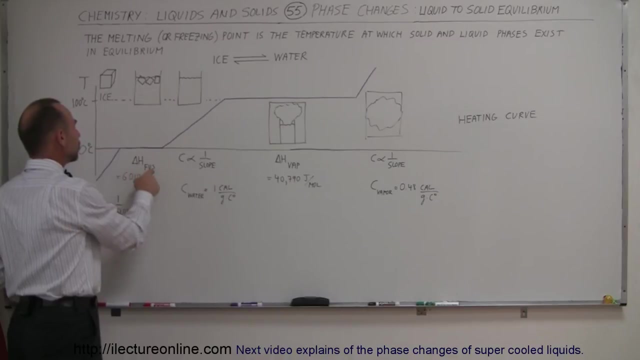 the water turns into steam. Notice, by adding the same amount of heat per unit time to boiling water, it takes a lot longer to boil the same amount of water as it took to melt the same amount of water. That is because the latent heat of fusion is. 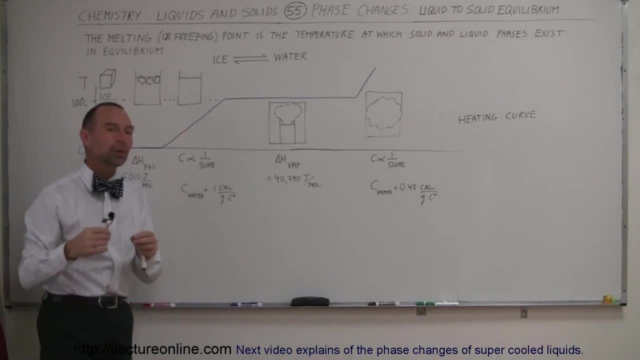 much smaller than the latent heat of vaporization. It takes much more energy to break away the molecules from a liquid than to take a set of molecules in a lattice state and making them random so that they start rolling over each other. so from a solid to a liquid, Notice, it's 6,010. 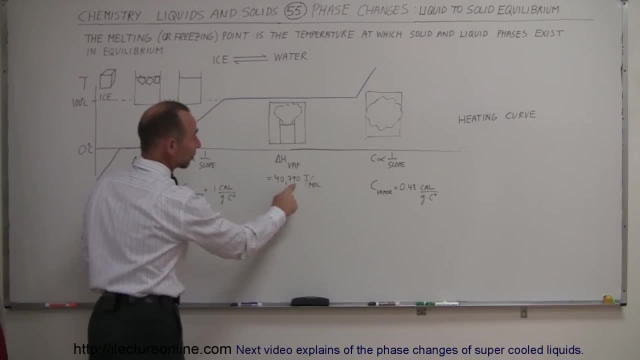 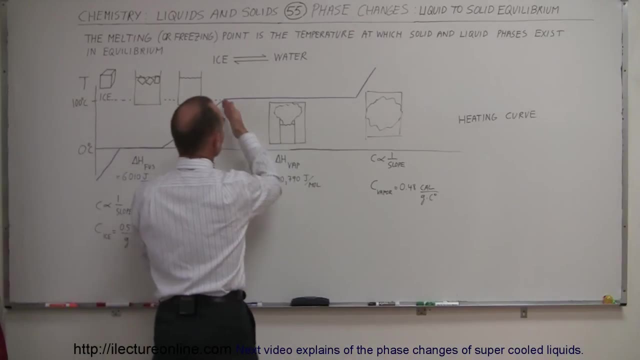 Joules per mole for the latent heat of fusion and it's an enormous 40,790 Joules per mole for the latent heat of vaporization. Then if you take all the liquid and completely vaporize all that liquid and you continue to add additional heat again at the same rate, then you can see that the 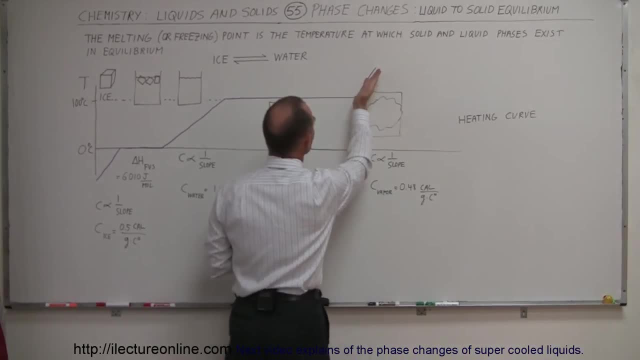 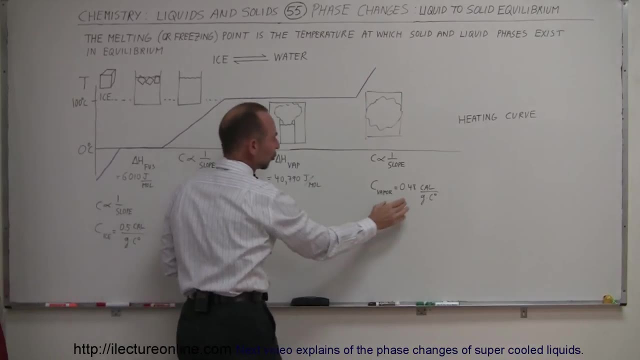 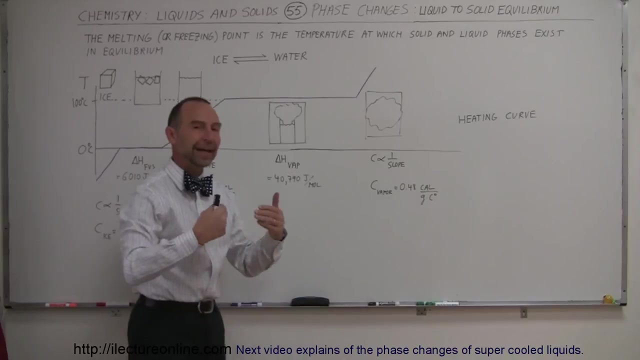 temperature begins to increase on the vapor right here. This slope is deeper than this, which would imply that the specific heat of vapor is less than the specific heat of water. and sure enough, this vapor is only 0.48 calories per gram per centigrade degree, and therefore the curve is on steeper. add. 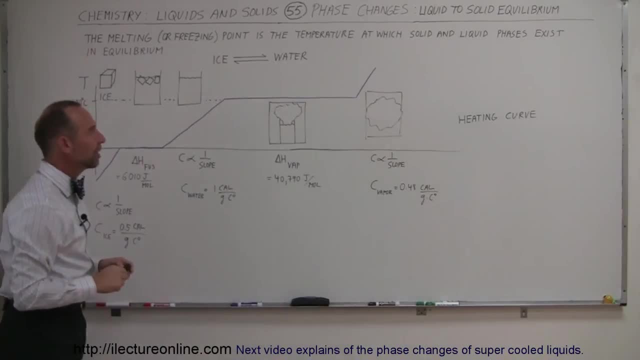 more heat to it, quickly rising the temperature of steam. so this is considered a heating curve. and when we talk about the liquid to solid equilibrium is the very interesting situation right here where, as we continue to add heat, after the ice has reached a temperature zero degrees, you can see that the water, the ice, will not increase in temperature any further. the ice 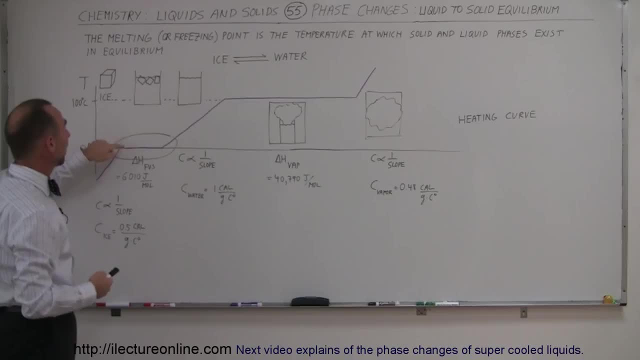 will begin to melt, it will change phase from solid to liquid and you can see that this will continue at an equilibrium temperature. that's why they like to work use the word equilibrium. it's an equilibrium temperature until all the ice has melted before any of the water begins to increase.